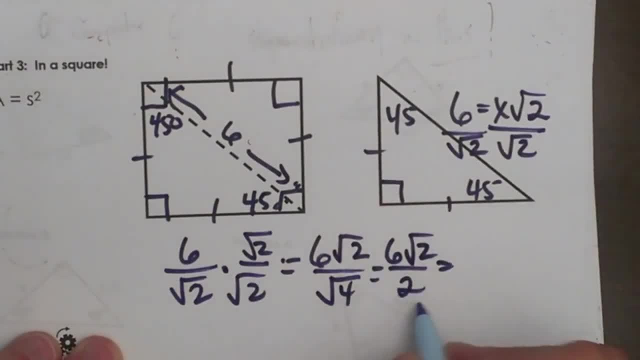 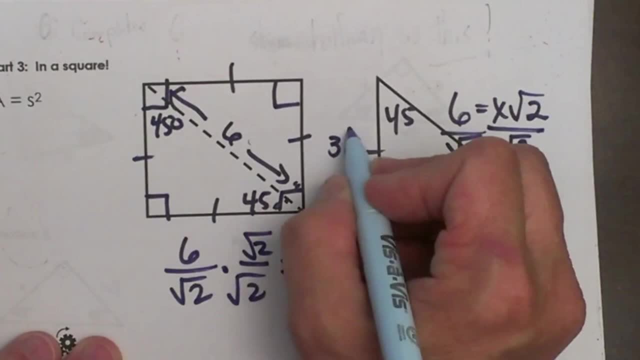 So that is 6 root 2 over 2, which again reduces to 3 root 2.. So that is the side right here. So I have two legs that match 3 square root 2 and 3 square root 2.. Now I can just plug it into my formula. 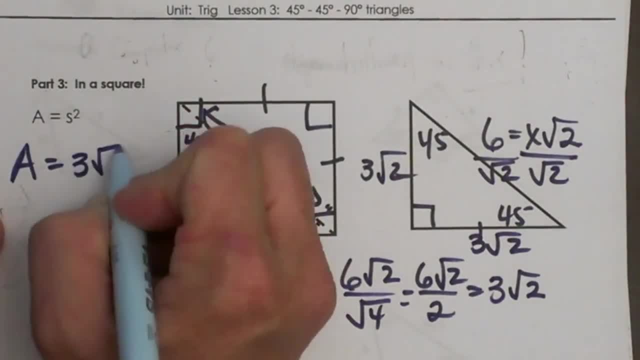 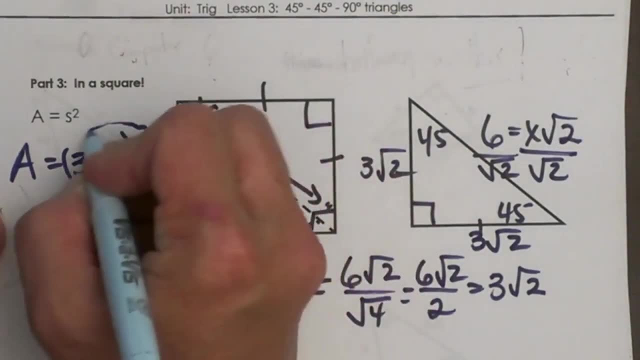 To find the area. I take 3, square root 2, and I am going to square the whole thing, not just squaring the square root but also squaring the 3.. So you have to kind of like distribute, We have to square the 3 and square the square root of 2.. 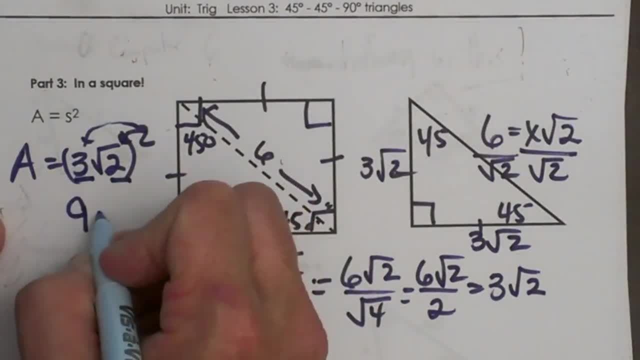 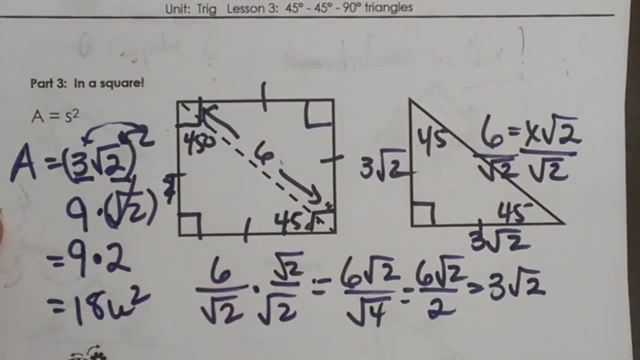 So 3 squared is 9, and the square root of 2 squared that just cancels out, so you get the square root of 4. Which is just 2.. So 9 times 2, so the area is going to be 18 square units and that is how you find the. area of a square, given the diagonal. 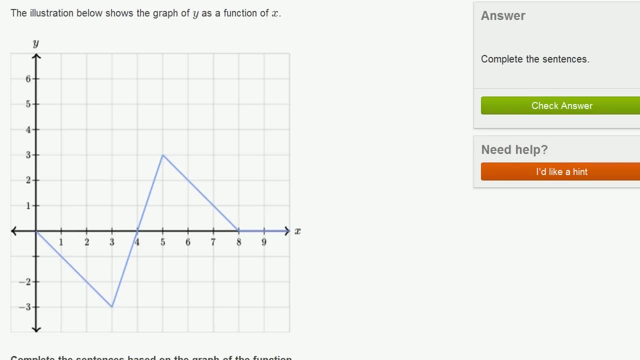 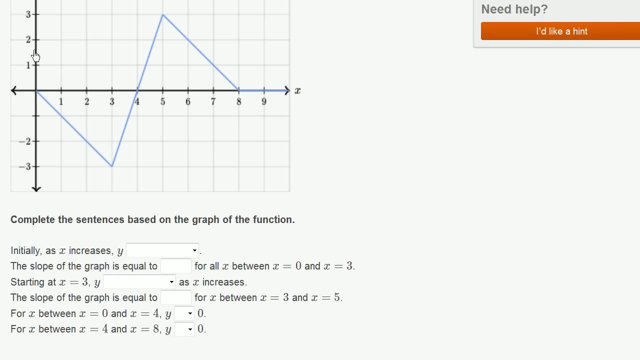 The illustration below shows the graph of y as a function of x. So that's this graph right over here. And then they start to ask us some questions. Complete the sentences based on the graph of the function. So this x is our y-axis, our vertical axis. 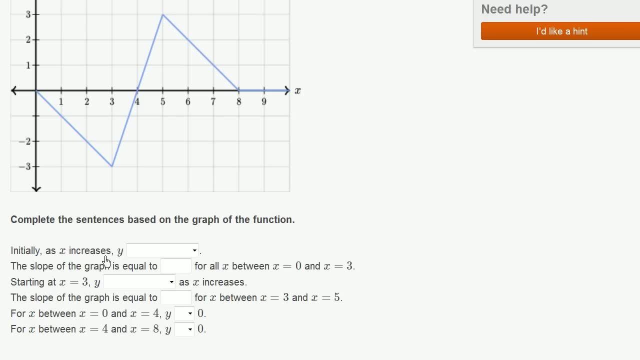 Horizontal axis is x-axis Initially, as x increases. let's think about it Initially. so when we start from x equals 0 and x is increasing, what's happening to y? Well, y is decreasing, So y decreases. So as x increases, initially, y decreases. 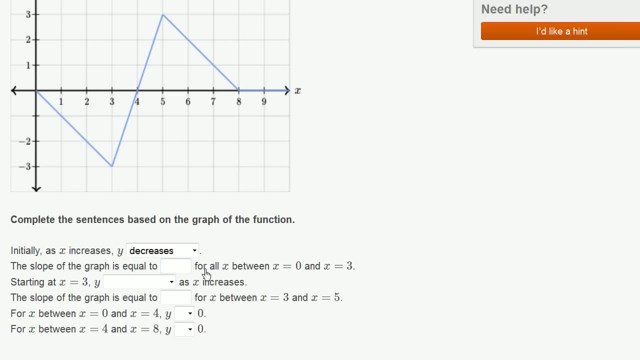 The slope of the graph is equal to blank, for all x between x equals 0 and x equals 3.. So x equals 0 and x equals 3, what's the slope? Well, every time we move 1 in the x direction.